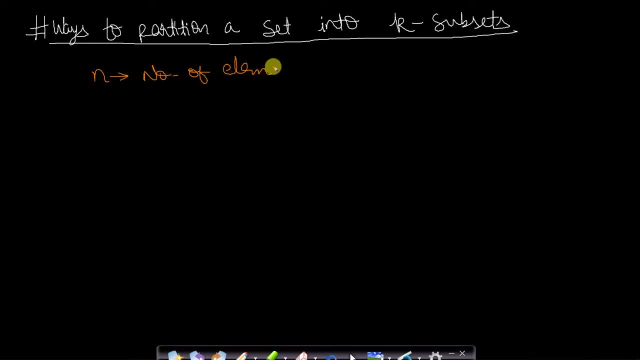 n as the number of elements. okay, and all the n elements are unique. All the n elements are unique. and you want to divide these n elements into, let us say, k number of subsets. okay, So this k are the number of subsets. Let us now take an example in order to get a better understanding. 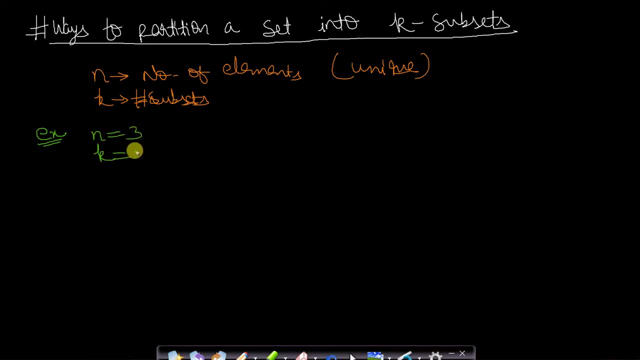 So let us assume n is equals to 3 and k equals to 2.. That means we have three elements, three unique elements, and we want to divide these elements into two number of subsets. Let us say our element is 1,, 2 and 3.. So in how many ways can we divide? 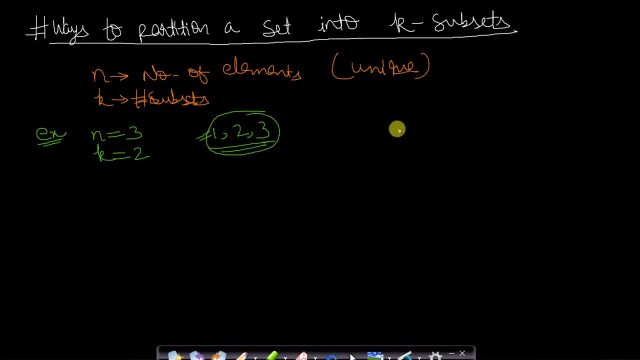 these n elements into k number of subsets. So let us assume n is equals to 3 and k equals to 2.. These three elements into two number of subsets. So if I take 1,, 2 in one subset and 3 in another, 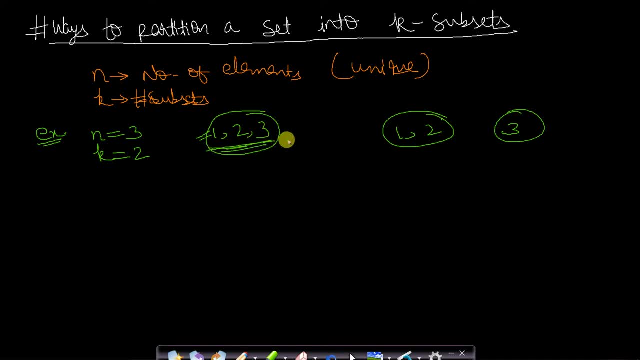 subset, then I have divided this element- 1, 2 and 3- into two number of subsets. So this is our first way. okay, So this is our first way. One another way can be if I take 1, 3 in one set. 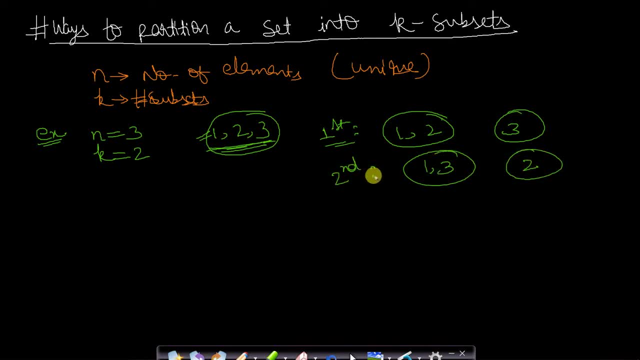 and 2 in another set. okay, So this is our second way. One still another way can be: if I take 2, 3 in one set and if I take 1 in the second set. okay, So this is the third way and there is no. 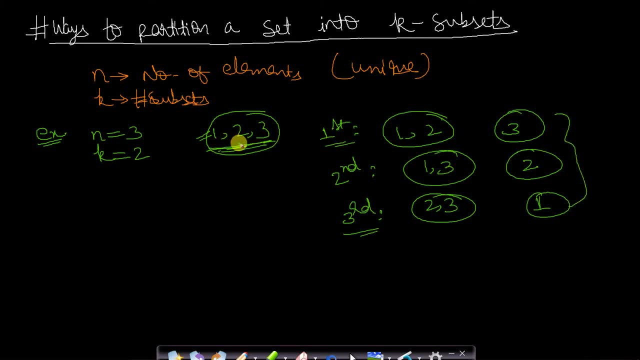 other way. okay, So we have divided our elements 1, 2 and 3 into two number of subsets in three ways. okay, So this is three ways. So this is our problem. statement, Given the value of n and k, where n is. 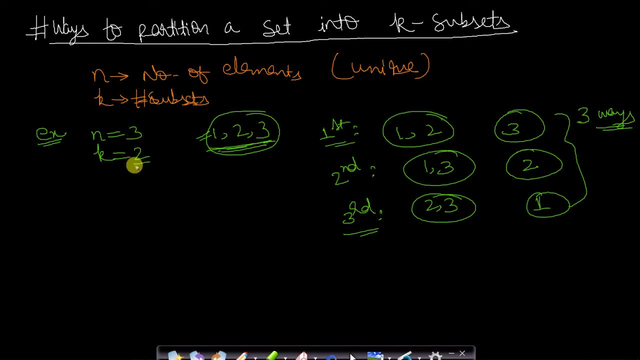 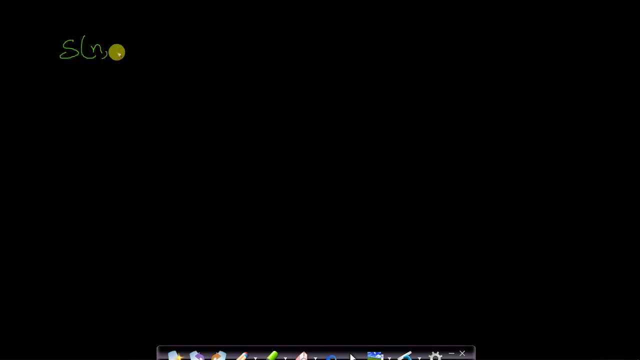 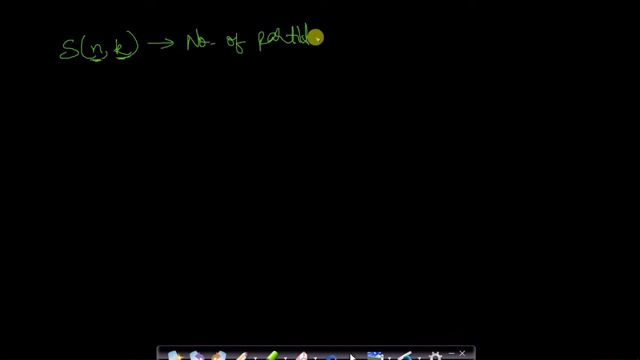 means the number of partitions, number of partitions of N elements. okay, number of partitions of n elements into K sets. so this is the meaning: number of partitions of N elements into K sets. this is the meaning of s of N, comma, K. so, given the value of N and K, how can we find the solution? how can we find the number of? 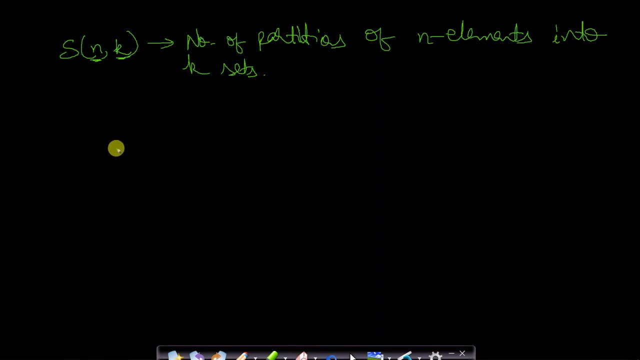 ways. so there is a recursive formula. let us first look at the formula and then we will get the understanding behind it. okay, so s of n comma k is equals to k into s of n minus 1 comma k plus s of n minus 1 comma k minus 1. okay, so let us first look at this part. so what does this part means? 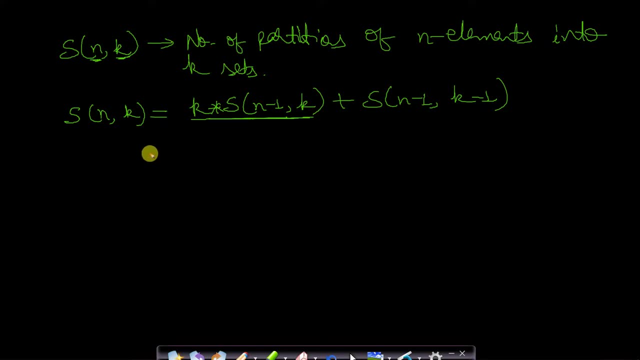 if you have n minus 1 elements and it is divided into k- number of sets. okay, so let me write the number of sets. let me take the number of sets to be case. okay, so these are the number of sets, and these n minus 1 elements are divided in k number of sets. okay, so where will the nth element go? 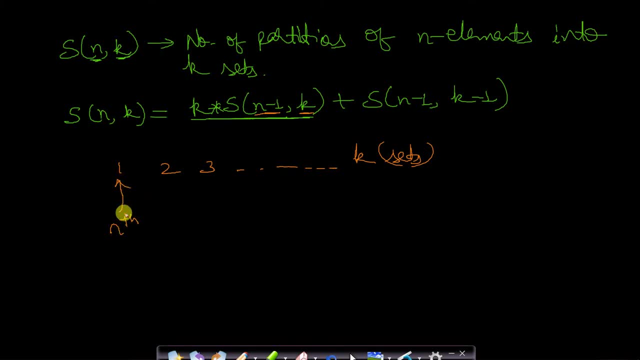 the nth element can go either in this first set, in the second set, in the third set, and so on. incidentally, it can also go in the kth set, okay. so there are k number of possibilities. okay, there are k number of possibilities for a given nth element to go and stick to a given set. okay. so that is why. 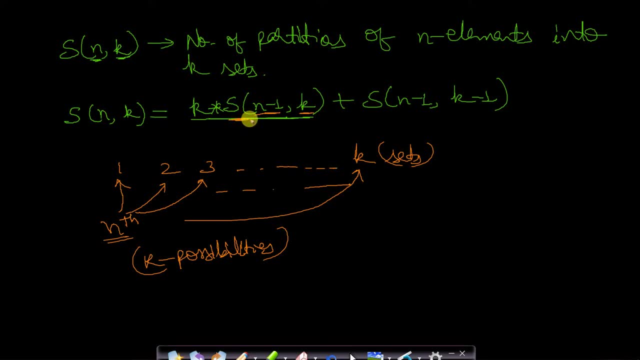 if we have already found the number of ways in this formula s of n minus 1 comma. k means that if you have n minus 1 elements and k number of sets, then in how many ways can you divide this n minus 1 elements into k number of sets? if you have found this answer, then the nth element can: 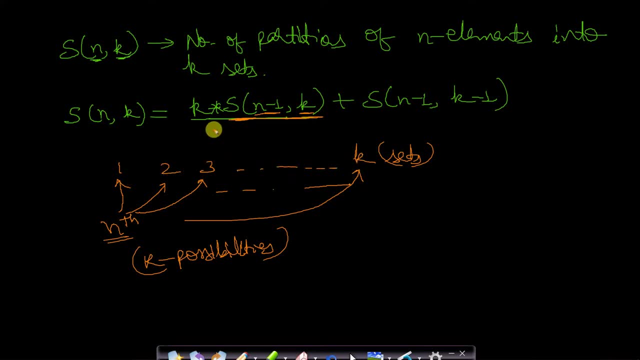 go and sit in any one of these k sets- okay, and that is why we have multiplied k with the solution of this element. okay, now this nth element can also go and sit to a new set. the nth element can go and form a completely new set- okay, where only one element will be present. so that is why we 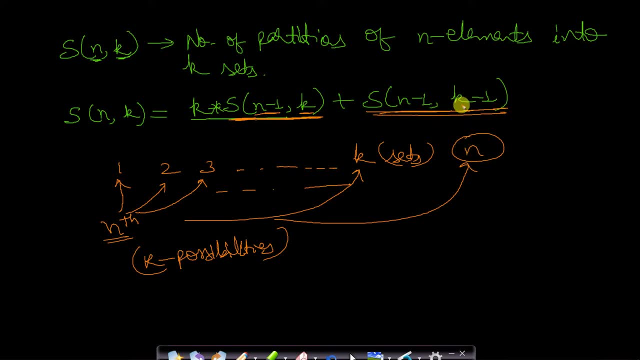 have included this one as well. this is saying that we had k minus 1 sets, okay, and we had n minus 1 elements, and by adding this nth element into a new set, the number of sets have become k- okay, and the number of elements have become n, and in this case this will not hold true, okay, so i hope. 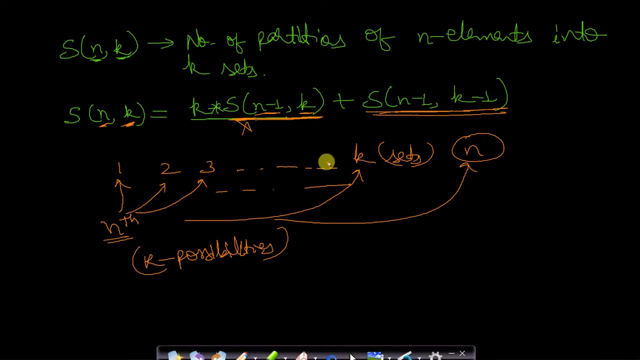 you are getting an intuition about it. it is very intuitive. if you think deeply and if you try it, then you will get a better understanding about it. okay, it is just saying that if you have k sets, then this nth element can go and sit in any of these sets. that is why we have multiplied k. 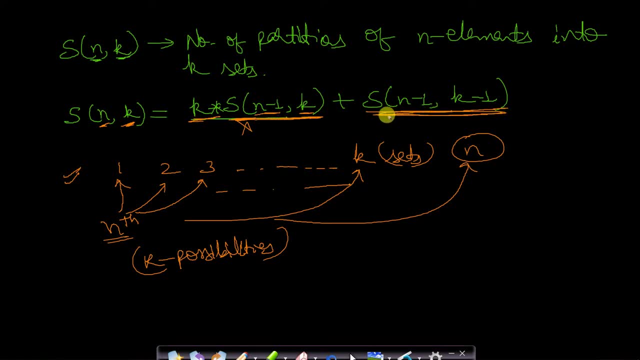 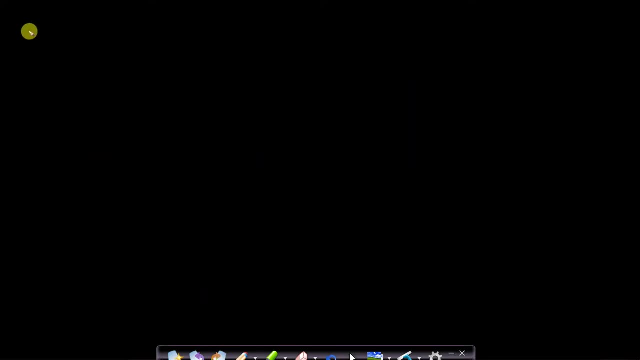 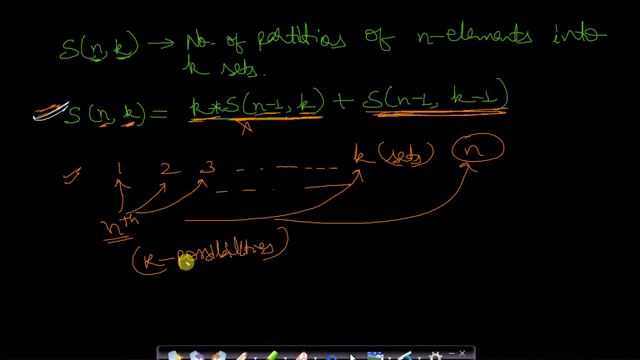 with this part, and this part is given if the newly added element forms a completely new set. okay, now let us look at the recursive solution. okay, so the recursive formula is the same as we have seen in the previous case. this is our recursive formula. okay, so we will use it here. 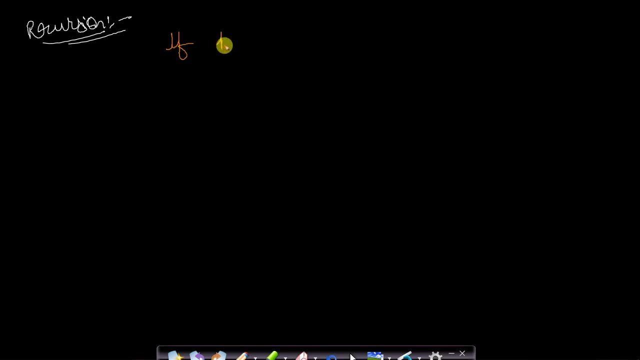 in our recursive code. the base condition should be: if k, that is, number of sets, is equals to 1, then we will have to return the value 1, because if there is only one given set, then all the elements, whatever it is, will come and fall in this single set, and so there will be only one possible way. 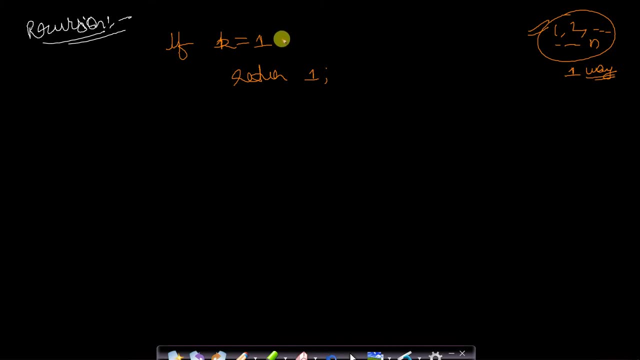 okay, because we cannot arrange it in any other way. or if the number of sets is equals to n, then also we will have to return the value 1, because if there is only one given set, then all the elements, whatever it is, will come and fall in this single set, and so there will be only one possible way. or if the number of sets is equals to n. 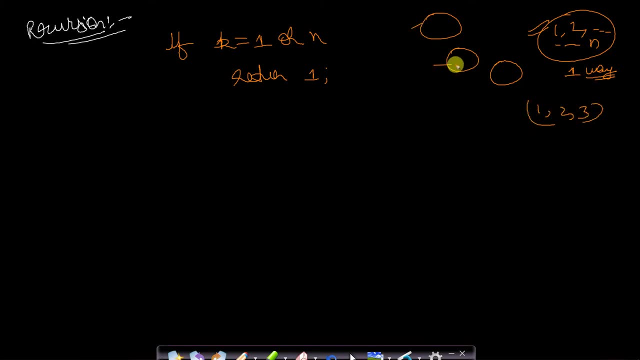 let us say we have 1, 2 and 3 and if the given sets are also 3, then if we fill it in in a single way, then we cannot just change the numbers and make another way, because arrangement do not matter here, it is only the content of the set. okay, if you write 2, 1 and 3, and if you write 1, 2 or 3, it won't matter. 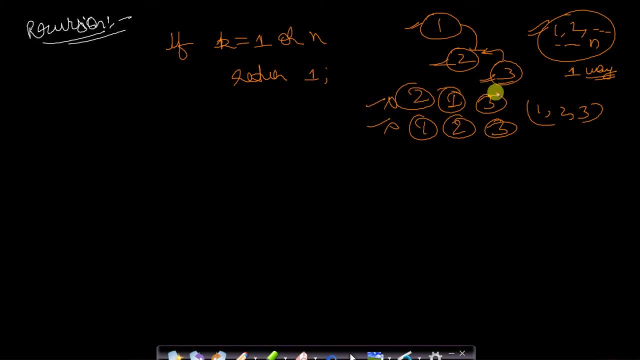 both are same. okay, because the arrangement is the same. so we will have to return the value 1, because if the number of sets is equals to n, it is only the content of the set. okay, so that is why this is our base condition and what will be our recursive solution. 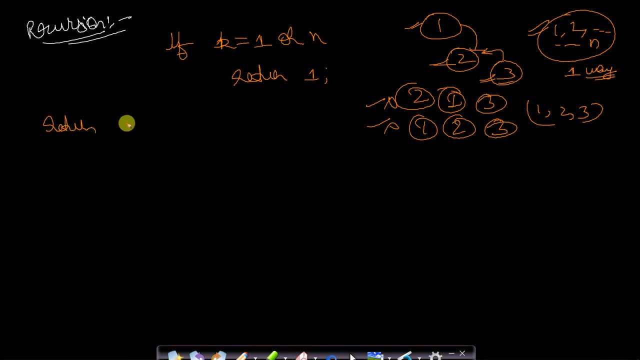 after this if statement: we will write return k into s of n minus 1 comma k plus s of n minus 1 comma, k minus 1. okay, and that was our recursive code. if you can remember, this was our recursive formula. this entire process is the recursive code. so we will write return k into s of n minus 1 comma k plus s of n minus 1 comma, k minus 1. 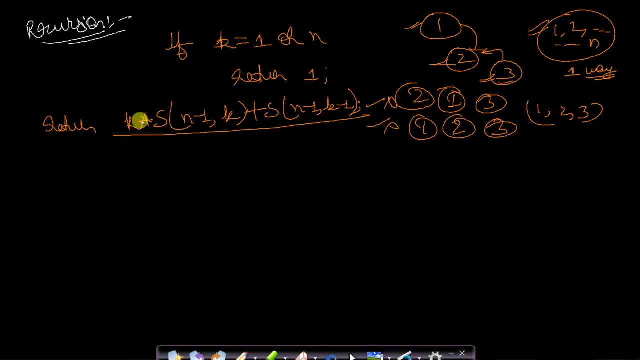 thing and this we are using it here. okay, this s is our function name, so this function is basically s. here it is taking two parameters: n and k. okay, so this is the recursive approach. this has exponential time complexity. okay, so the time complexity here is exponential because we are doing the same work. 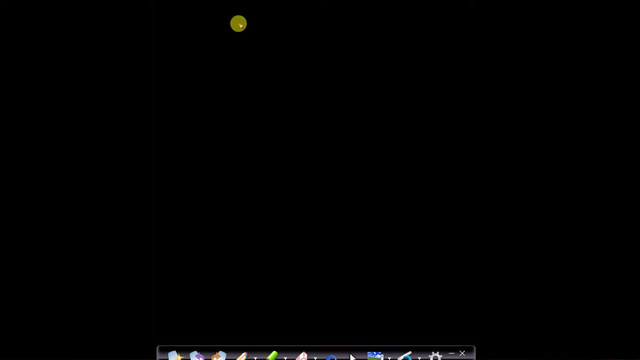 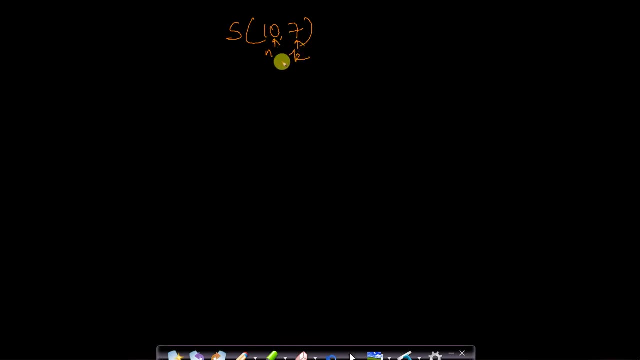 elements is 10 and number of sets is 7. okay, so s of 10 comma 7 can be written as k into okay, k into s of n minus k, that means 9, and then k, that means 7. so this will be replaced by 7 plus. that will be s of n minus 1, k minus 1, okay, so this will be the formula. so that is why. 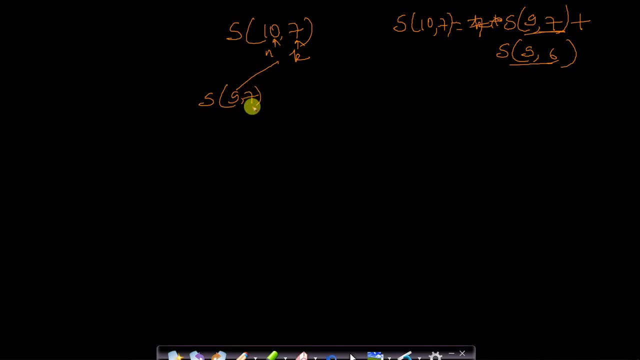 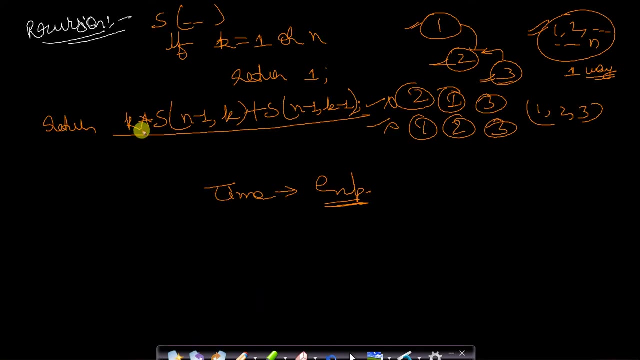 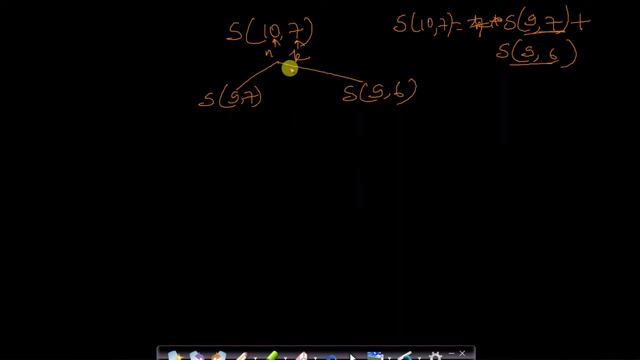 this will be divided into two branches: s of 9 comma 7, and the right branch will be having s of 9 comma 6. okay, because we were making two calls at each time. we were making two calls: s of n minus 1 comma k and s of n minus 1 comma k minus 1, and we are given initially the values of n comma k. 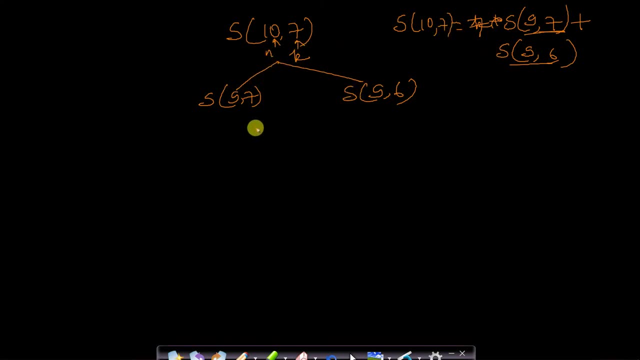 so that is why we can find the left and the right recursive calls. similarly, for this case, we can find that it is s of 8 comma 7 and this is s of 8 comma 6, okay, and this will go on. this will go on. 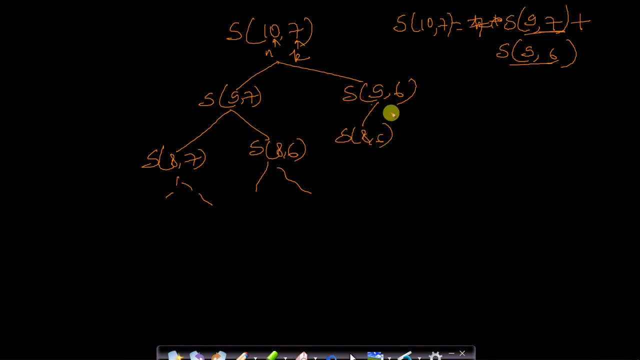 similarly for this case, it will be s of 8 comma 6, and this will be s of 8 comma 5, and this will also go on. okay, you can see that this one and this one is the same sub problem. they both are the same. 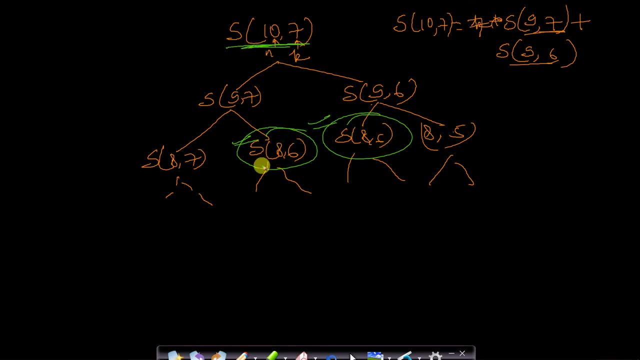 sub problem of this problem. okay, so we are computing this sub problem again. okay, and there are many other sub problems which we are computing again and again. okay, we are doing the same work again and again. therefore, the time complexity will definitely be exponential, okay. so how can we improve on the time complexity? we can improve by using dynamic programming. so 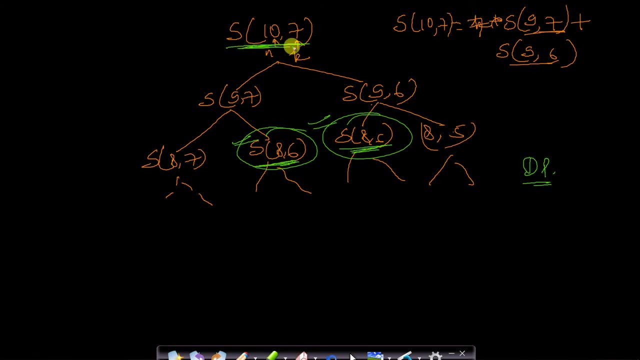 let us see if we can apply here dynamic programming. this entire problem is divided into sub problems and by solving these sub problems, as you can see in this formula, if you can solve this s of n comma 6 and s of n or s of 9 comma 7, then you can definitely solve this. 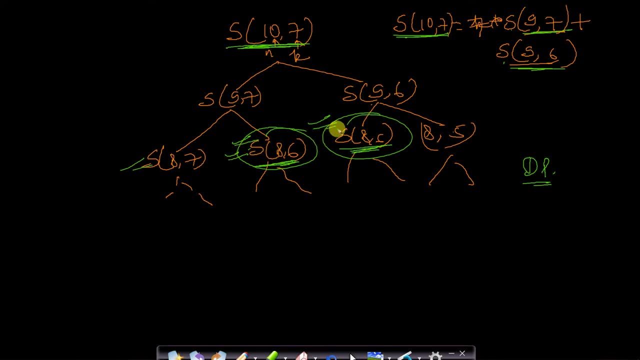 s of 10, comma 7. so solving the sub problems will yield the result to our problem. okay, and so it has a property of repeating sub problems as well as optimal substructure. optimal substructure because if we solve these sub problems in the optimal way, then the problem will also get solved in an 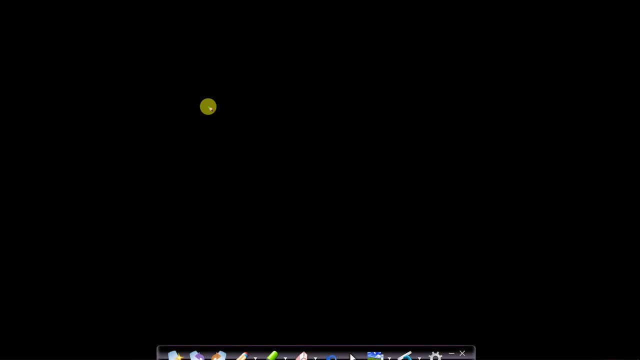 optimal way. so let us see how can we solve it by using dynamic programming. okay, so let me take n is equals to 4 and k is equals to 3. okay, and let us see how it is done. so i will just make a table of: let me write a dp of n plus 1 and here k plus 1. 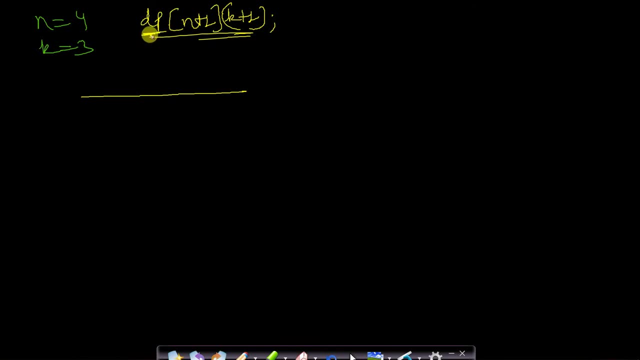 okay, this will be the size of our table and the table name. let us say it is dp. okay, let me write dp. okay, so the one in the below are the number of elements, this n is the number of elements and this k is the number of sets. okay, so let me draw the lines. okay, and now what we will do is we will. 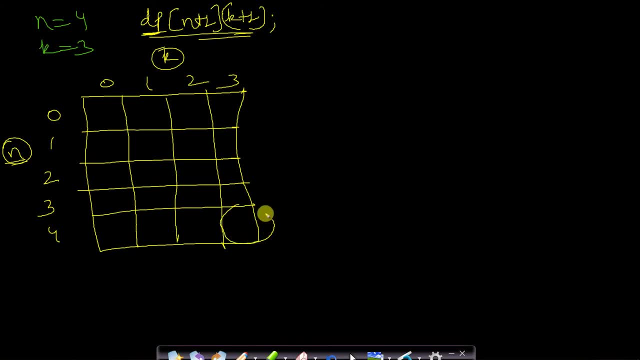 start filling this table, and whatever comes in this region will be our answer. okay, so, first of all, if you have no element, then you cannot form any set. so so this will be zero. and if you have any elements, but if you have no set, this zero means you don't have any set- then also there will 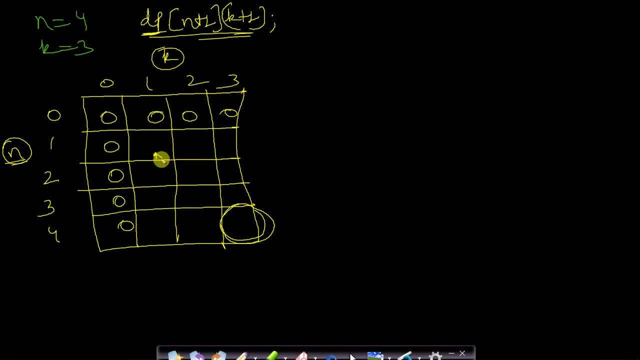 not be any possible way. okay, so that is why we will start from this point. okay, so let me write the code initially, so that you can get a better understanding. so it will be for i equals to 1 to n, and this will increase in steps of 1, and then we will need another loop. this loop is for these: 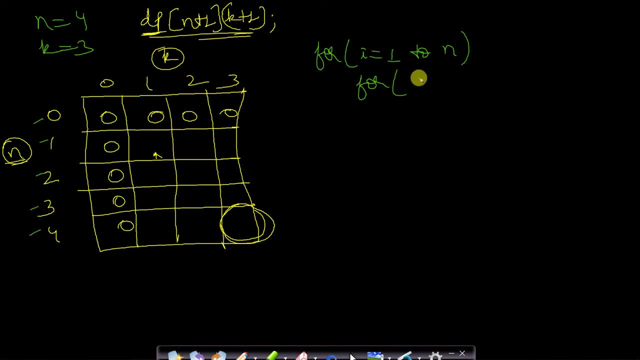 rows. okay for completing these rows, and we will know and we will need another loop for the columns. so that will be: j equals to 1 to less than equals to i. j equals to 1 to j. less than equals to i, and this will also increase in steps of 1. okay now if j equals to 1 or i equals to j. if this is the case, 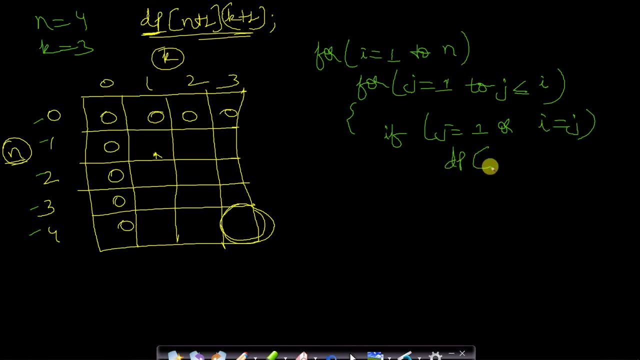 if any of this is true, then we will fill there. dp at i, j will be equals to 1. and why is that? because if we have only one set- this we have already seen- if we have only one set, then we can have only one way, okay. or if the 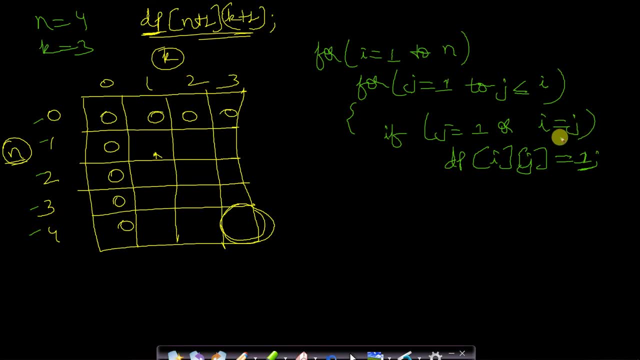 number of sets is equals to the number of elements, then in each set we can fill only one element, and that is why we will have just one way. these were the base conditions. if the base condition is not true, then what we will do is we will write our recursive formula dp at i. j will be equals to j. 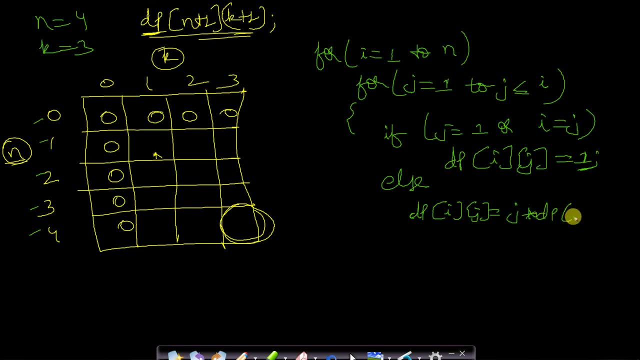 which is the number of sets into dp at i minus 1, into j plus dp at i minus 1, into j minus 1. okay, so this is our solution. let me fill this table and show it to you how it's done. initially, this first row and first column is zero, and then we will write our recursive formula: dp at i- j will be. 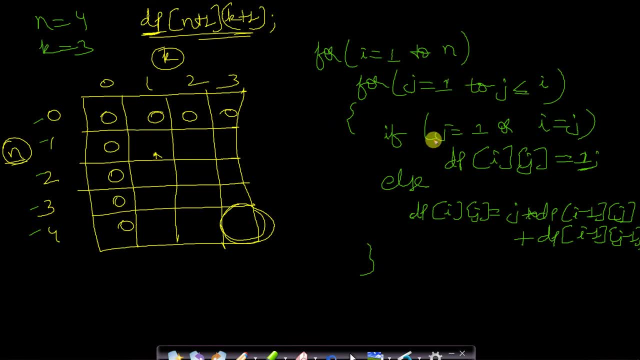 and we are starting from i equals to 1 and j equals to 1. ok, so this condition will be true. this condition will be true, and so here we will have 1. now, since j is less than equals to i and initially i is 1. therefore, j will break and the control will go to i. now i will 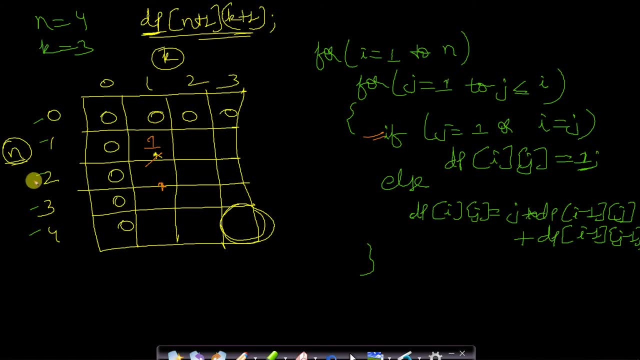 increment by 1, and so this will be our control. control will be in the second row. now j equals to 1, j equals to 1. that is why we will fill here 1. it will increment by 1, since i is now equals to 2. ok, now j is also equals to 2, and since i equals to j, therefore this condition: 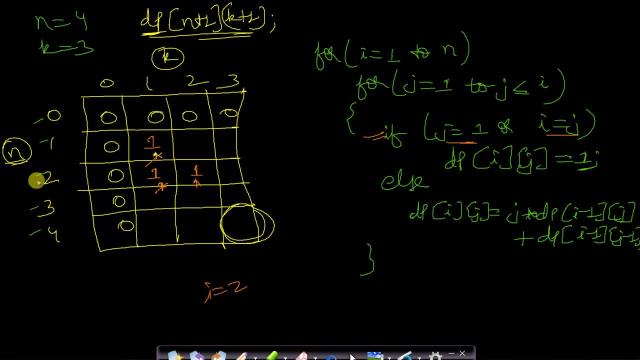 is true, and we will again fill it by 1. this is saying that number of elements and number of sets are equal. that is why we can have only one way. ok now, i will increase, i will break, j will break and i will increase. ok now. 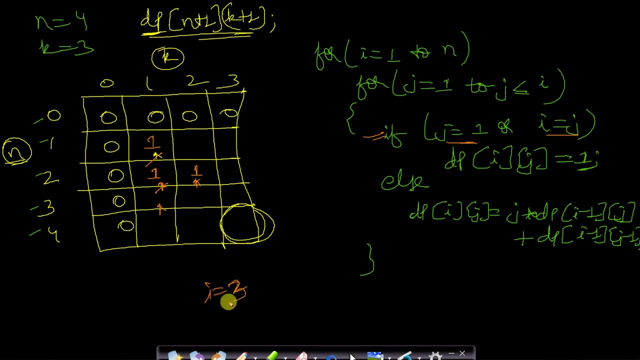 will go here in the third row. now j will again start from one, since j equals to one. therefore we will fill it one. why we are filling one here? because we are having only one number of set and since we are only having one number of set, so element, any element, whatever it comes, it will. 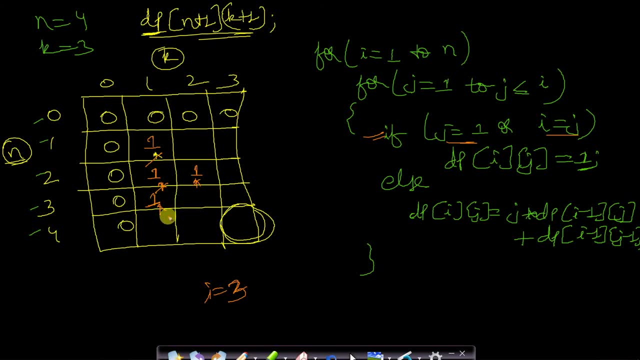 only fit in that set and therefore we will have only one possible arrangement of the sets. since we have only one set now, j will increase its value. now, i is not equals to j and j is also not equals to one. therefore, this condition will be true. the else condition will run. it is saying: 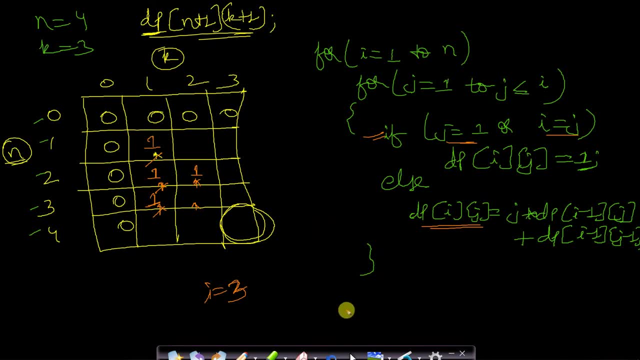 that multiply j. that means number of sets. here the number of sets is now two. and dp at i minus one j. dp at i minus one j is: this is this element. this is one, okay. and now add dp at i minus one, j minus one. dp at i minus one j is: this is this element. this is one, okay. and now add dp at i minus one j minus one. 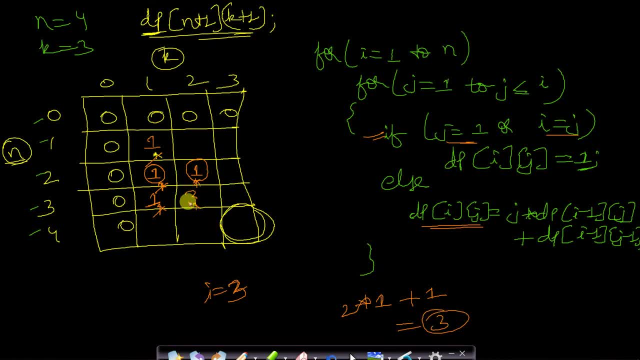 dp at i minus one j is this is this element, this is one. okay, and now add dp at i minus one, j minus one, this element, and this will become three. okay, so you will add, add and write here three. now j will increase. okay, j will increase. and since i is now equals to j, since number of elements equals to, 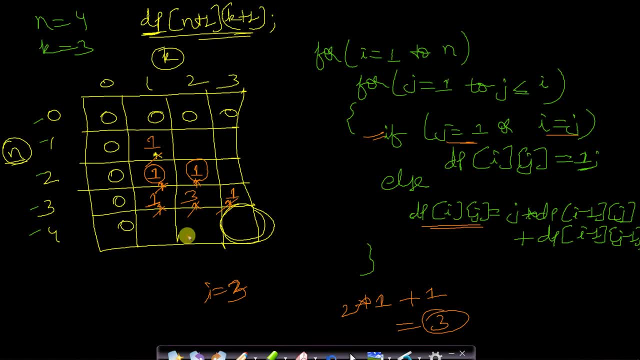 number of sets. therefore, we will write one here and now, j will break and i will increment to four. now j will again start from one and since j equals to one, therefore this will be one. now j will increment. okay, and we are reaching to. k equals to two. now, j is not equals to one. 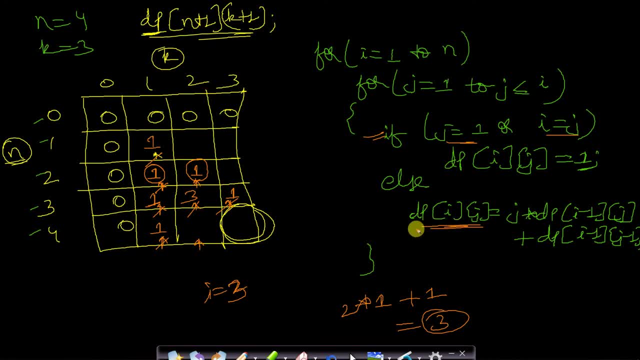 and i is not equals to j. therefore, we will follow this dp formula and what this will say. this says that multiply the number of sets. here, the number of sets is two. now, okay, because j equals to two. two into the diagonal element, this diagonal element, one plus add this element. 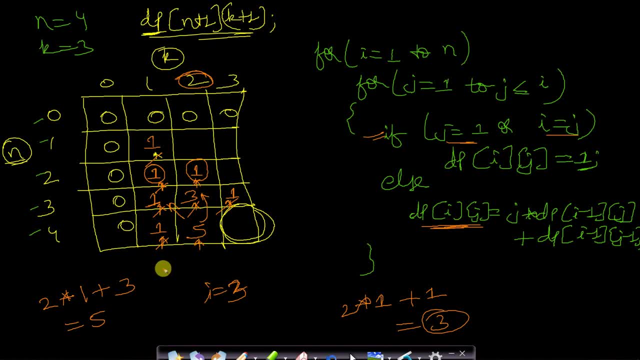 three, okay, and that will be equals to five, and right here, five. now we move on to the next element. okay, so the next element is: j equals to three. now, for j equals to three. this condition will not be true, okay, so the else part will run, and so the answer will be two into three plus one. that means 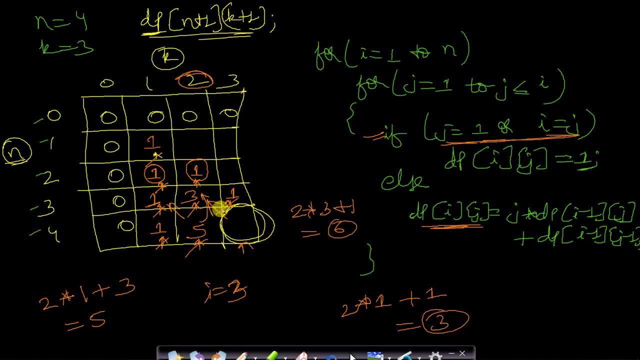 it will be six, because this is the diagonal element. this will be multiplied with two. we'll enter here and here you'll come six. so this is the dynamic programming solution. okay, so what is the time complexity? in this case, the time complexity is order of n square. 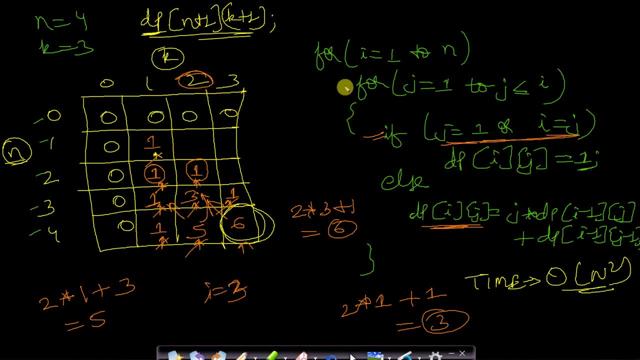 because we are building this table in order of n square time and you can see that we are using two loops. okay, and this will be order of n and this is also order of n, so you can say that it is order of n square. and what is the space complexity, since we are building this table? 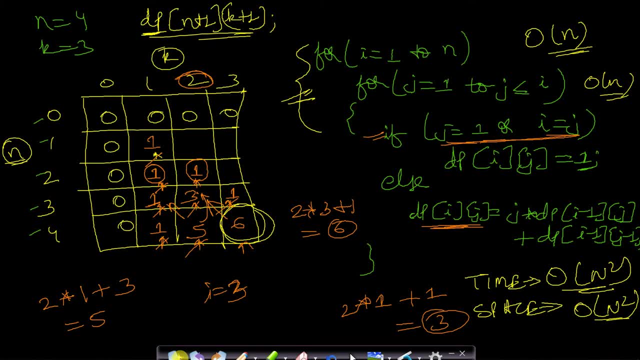 this is taking order of n square space. okay, there is still an optimization over this method. what is the optimization? as you can see that in this entire table, we are not requiring this table, but we just require only two elements. okay, only two elements at a time for a single element calculation. let us say for this: 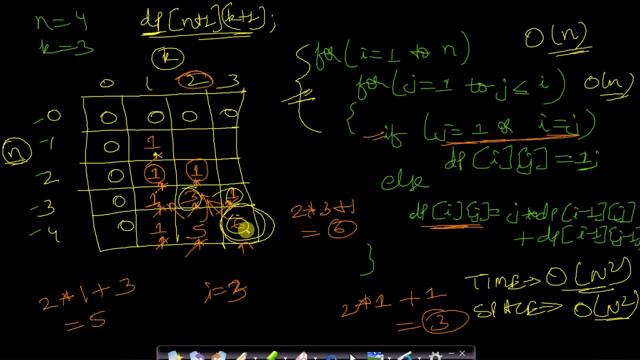 six, we require this three and this one in order to calculate this six. okay, and for this five, we just require this one and this three in order to calculate the value of this five. okay, so you can see that in order to calculate a row, we just need the value of the previous row. so at 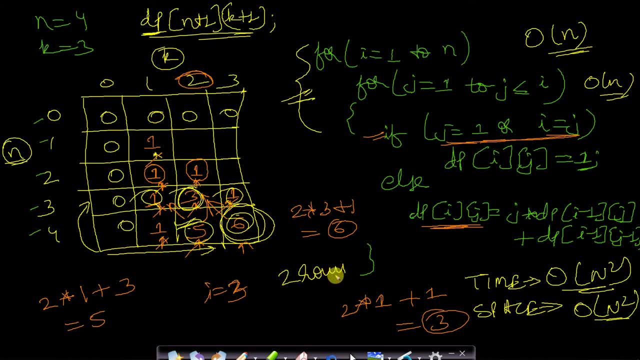 any time, you just need to store two rows. okay, at any time, you just need to store two rows. therefore, if you can optimize this problem, then the space complexity will decrease from order of n- square to just order of n. okay, so this will be good if you practice it. okay, so these are.